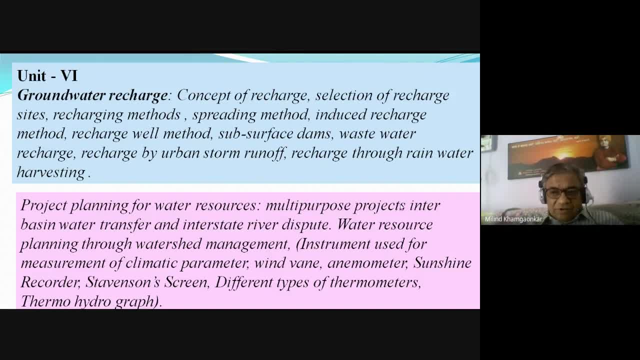 one purpose. earlier it was done. it was to be done that the project was constructed: a reservoir for the drinking purpose, for the hydroelectric purpose, only for irrigation purpose. like the pinch project at the Parshuni, it was earlier constructed for the irrigation purpose only. the two canals are there. 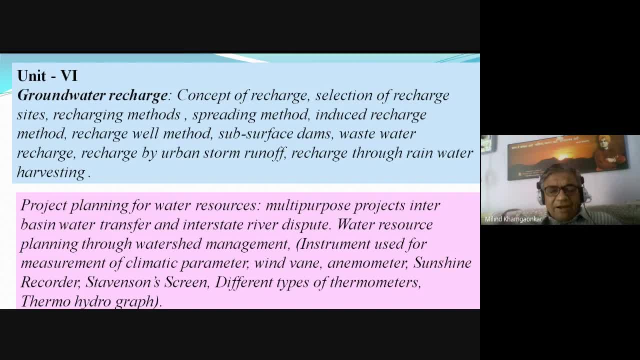 right bank canal and left bank canal and that canal was to supply the irrigation water for Nagpur district, Bandara, some part of the Garchi, Roli and Goondiya. but now, later on, as the demand of the drinking water from Nakpuri city arrived, then some of the water of the irrigation is being 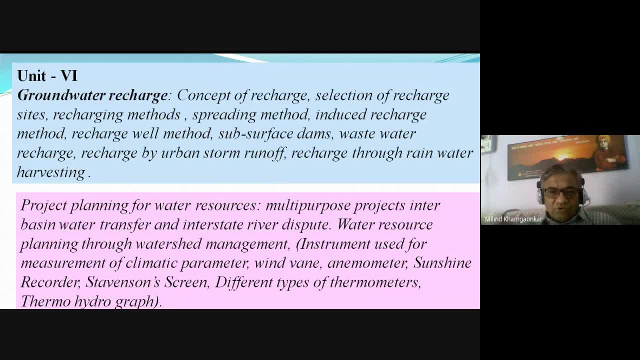 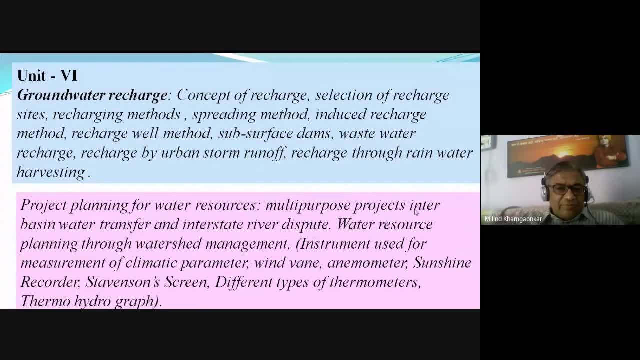 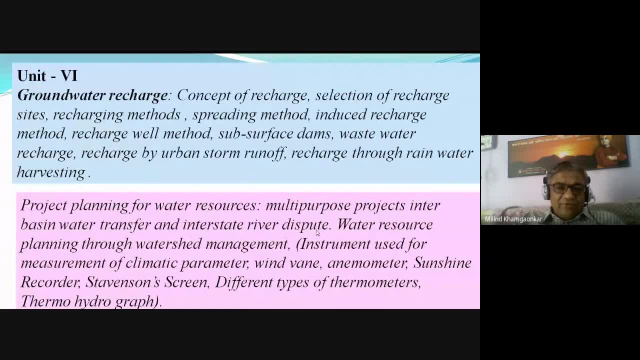 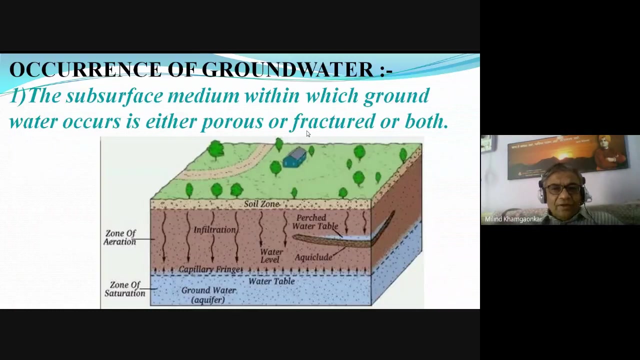 and jisco river linking projects and there are certain instruments. they are they. we want that you should know. so this is the syllabus of this unit. we have seen in our earlier unit, number 5, did that the groundwater occur below the surface of the soil and subsurface also of the soil, due to the nature of the soil, that is. 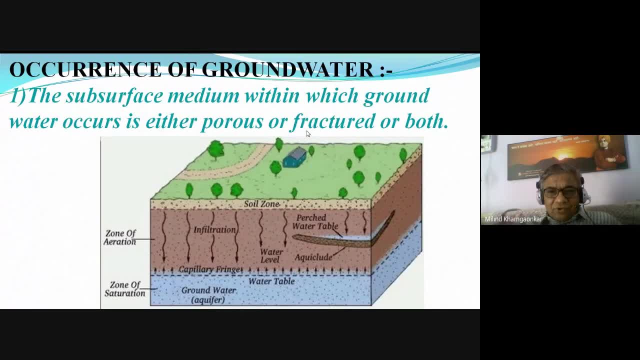 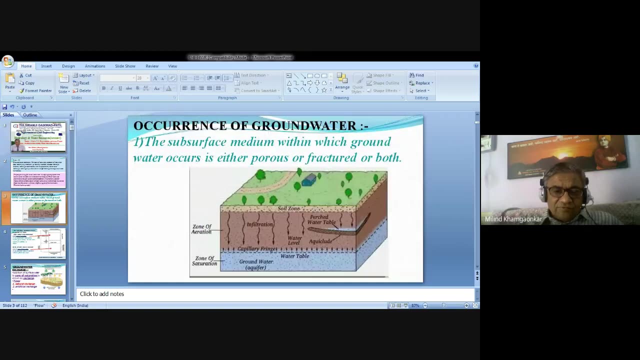 the porous nature of the soil or if the rock is there, then the fractured nature of the rock, or both porous and the fractured nature of the subsurface is the one is the cause of the percolation of the in percolation of the precipitated. 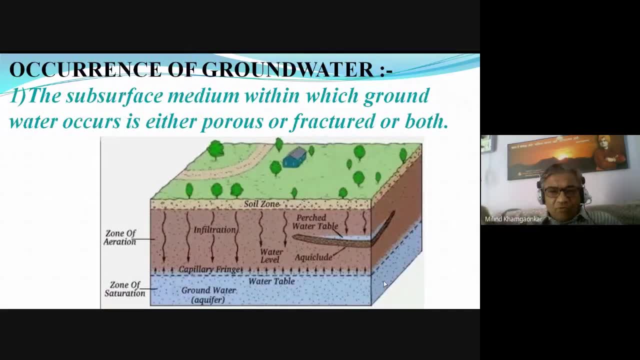 water and that percolation we have called as the innexpression, infiltration. this we have seen in our last lecture, in our last unit, how the groundwater occur and as it is the groundwater. groundwater means water which is available below the ground surface and the- if you go through this sketch, 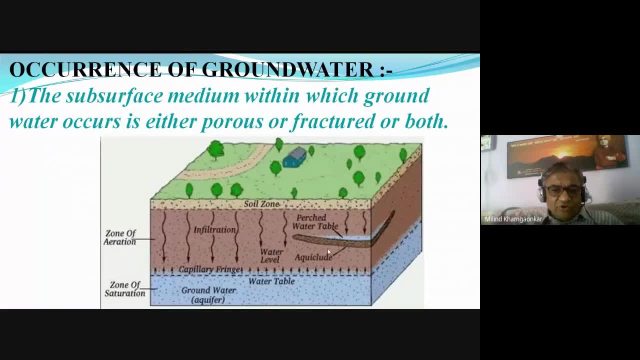 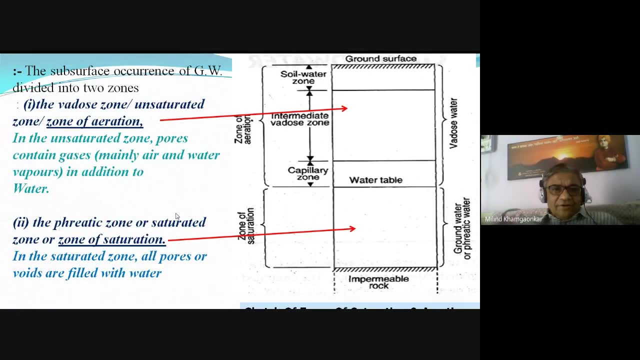 here you can see or you can revise what you learned in your last unit. and we have also studied that this sub surface where the groundwater occurs is divided into two zone. the first is the haddos, or the unsaturated zone, or the zone of aeration, the top zone below the ground surface. 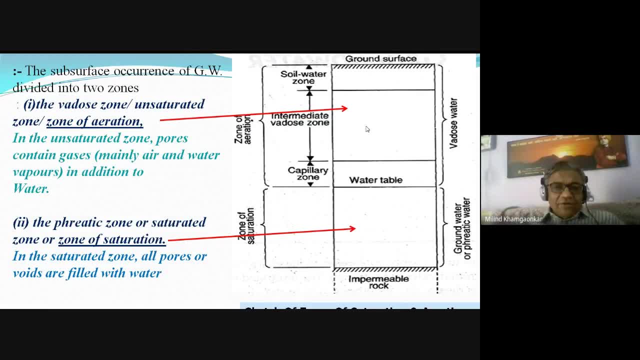 and the second zone where the groundwater occurs, and the third zone where the where generally, in the soil pores, in the soil voids, air is present and certain water vapour is present And very few quantity of the water is available in this vadoz zone or unsaturated zone, 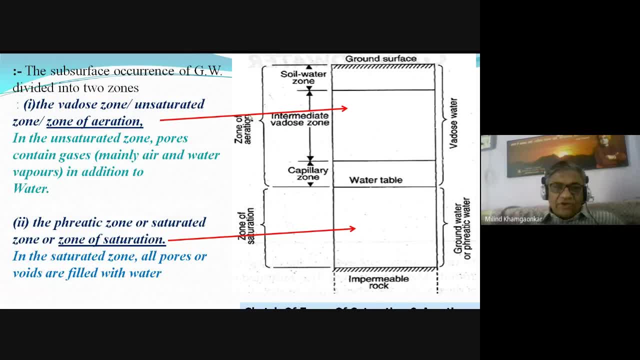 But below this zone of aeration- vadoz zone, or unsaturated zone- the another zone is available that is called as the phreatic zone, or saturated zone, or zone of saturation, where the water is abundantly available. If it is unconfined aquifer, then the water, the topmost surface of the water available, is the vadoz zone. 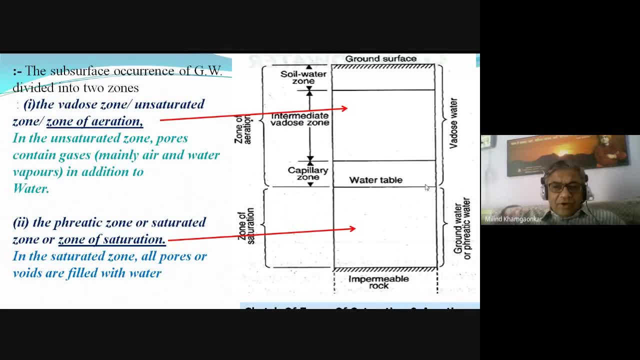 That is the top of that unconfined aquifer and the bottom, most part of the unconfined aquifer is impermeable rock. This we have studied. and also we have studied that for confined aquifer, that is, which is confined between two impermeable stratas. 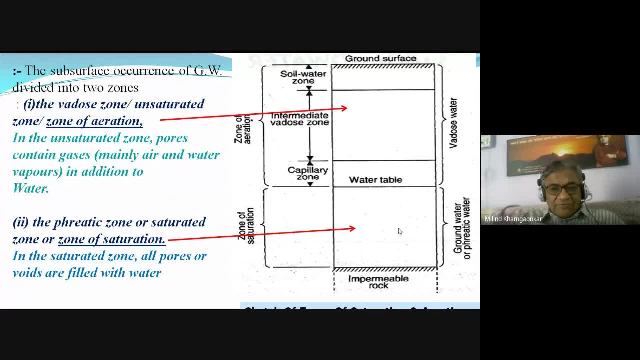 Again, aquifer means water reservoir Below the ground, So in confined aquifer, which is also available in the zone of saturation or the phreatic zone or the saturated zone, where in the pores of the soil water under pressure is available, 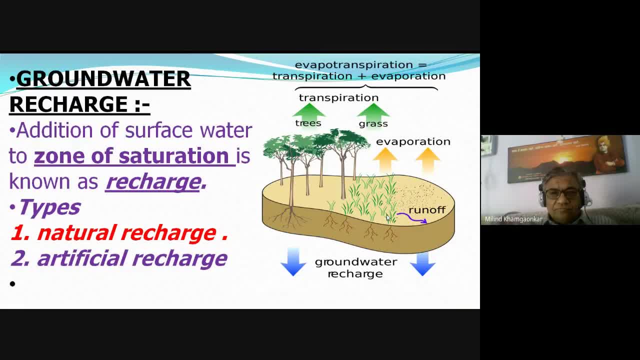 This bit revision we have done Now, where from this water Water comes into the confined aquifer or into the unconfined aquifer? That occurrence, Or that percolation, Or that addition of the surface water due to the rain or precipitation. 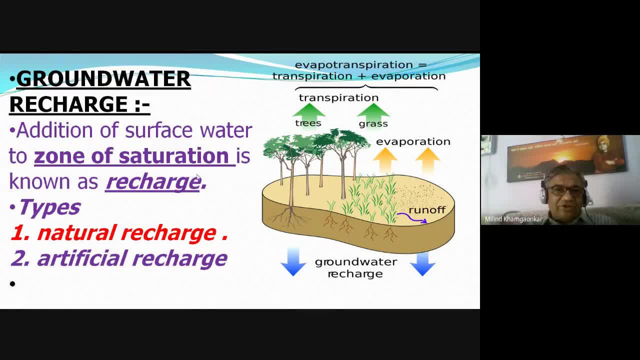 To this zone of saturation is called as the recharging of ground Water. The definition, That is, the adhesion of the surface water Do to the precipitation, To the zone of saturation, that is, to the unconfined aquifer as well as confinedth aquifer. 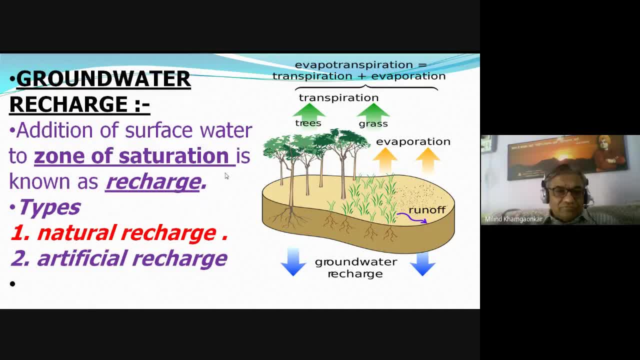 Is called as the recharging of the groundwater, Or recharge in short. This is not a difficult term, nor it is new. All this unit is a type of knowledge which is available to you. It is not new to you. Only thing is we are again recharging your knowledge, or we are again trying to refresh your knowledge. 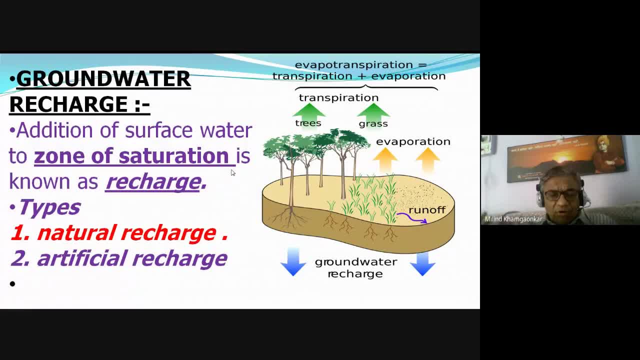 In scientific way. We all know what is groundwater recharge, what is rainwater harvesting, All these things we are very much aware of. Only thing is we are trying to understand it from scientific or technological manner. So this groundwater recharge, as I have just told you, is nothing but the addition of the surface. 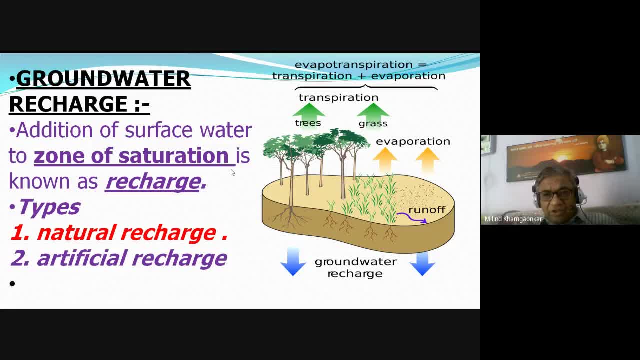 Water Again, from where the surface water comes. the surface water comes from the precipitation or the rainfall. That is, addition of the surface water from the precipitation or rainfall to the zone of saturation is called as the recharging of the groundwater. And what is zone of saturation? Just now we have tried to revise it. 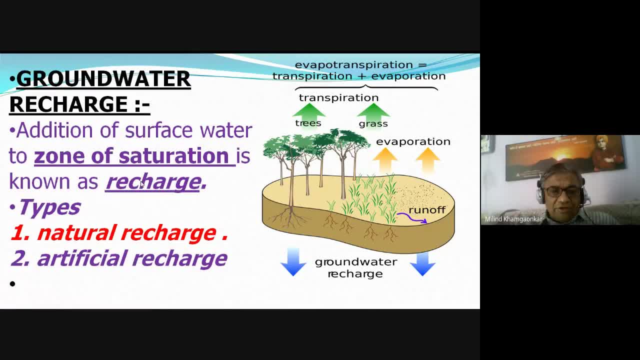 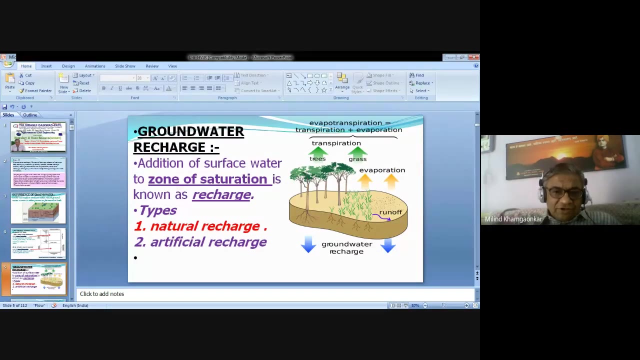 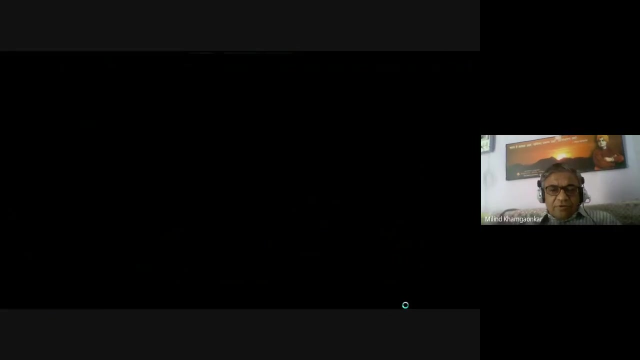 Now this recharging of the groundwater Is done in two ways, or if there are two types of the groundwater recharge, The first is natural recharge and the second is artificial recharge. The first is natural recharge and the second one is the artificial recharge. You can see here: 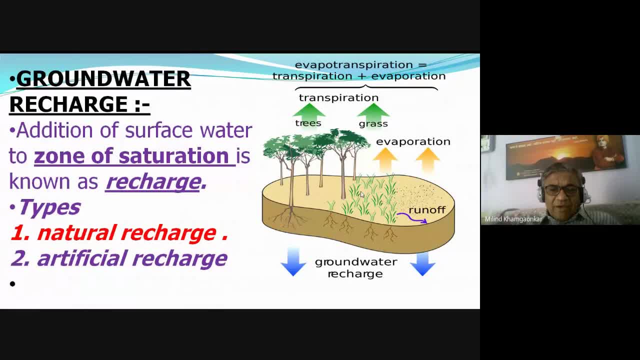 On the right side, as per my regular practice. I try to show by the sketch or by certain photograph. all hydrological cycle is shown here from unit one. we are trying to understand and whatever water that infiltrates from the precipitation. after the infiltration the water moves below the precipitation. 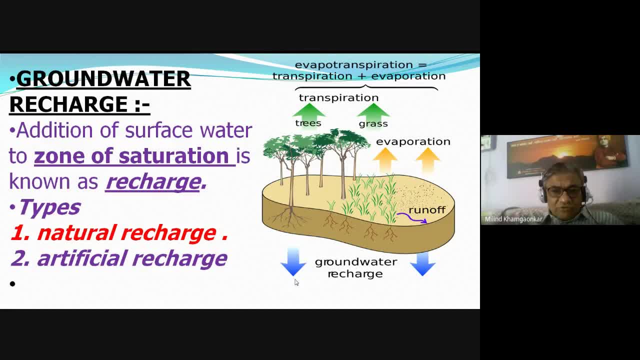 They move The ground surface into the ground surface due to the gravitational force And also due to certain surface tension and the capillary action into the pores of the soil. Move downwards Reaches to the own confined Or reach us to the confirmed activity. 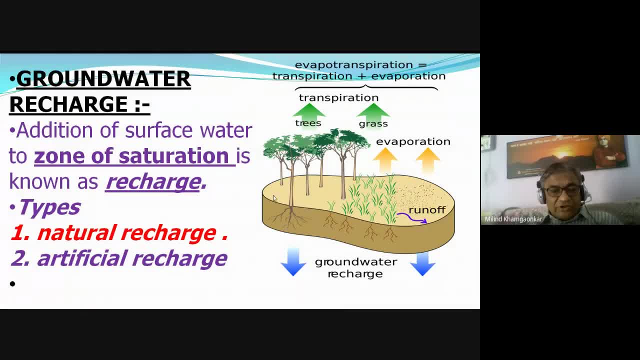 For also, at certain, when the water percolated from certain locations We are REALLY, they get into The ground. Its the unconfined aquifer meets the ground surface and in this way, these two aquifers, that is, the unconfined and the confined aquifers, get the rainwater. why? 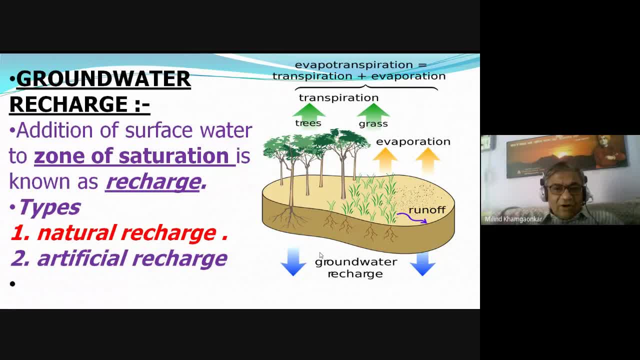 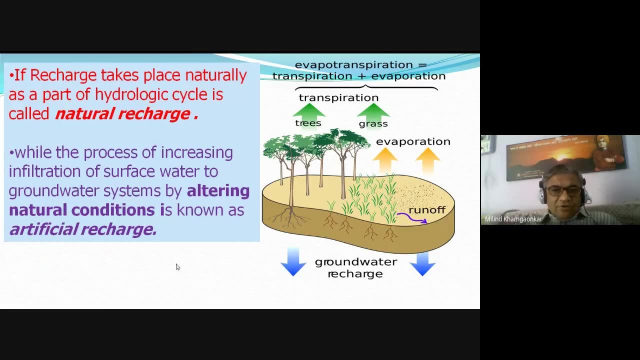 a percolation or infiltration and they call it and they get recharged. so this recharging is done by the two ways: that is, natural and the artificial recharge. so when this recharge of the groundwater takes place naturally as a part of hydrological cycle, then it is called as the natural recharge. we have seen the 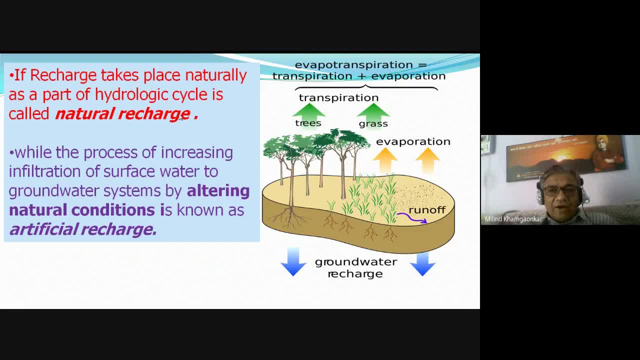 various components of the hydrological cycle, from evaporation to again runoff and the re-evaporation: evaporation to evaporation: evaporation, formation of the clouds, transportation of clouds due to the winds. condensation, water drop formation or the rainfall or the precipitation formation: formation due to the condensation of the nuclei and then precipitation. 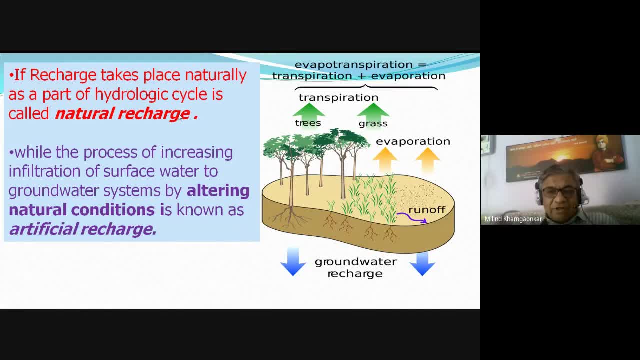 occurs over the ground surface, then infiltration, infiltrated water against converts into the two runoffs, that is, the subsurface and the base water, or the groundwater flow, and this groundwater flow is nothing but the groundwater recharge. when all this takes place now, in this natural way, in this hydrological 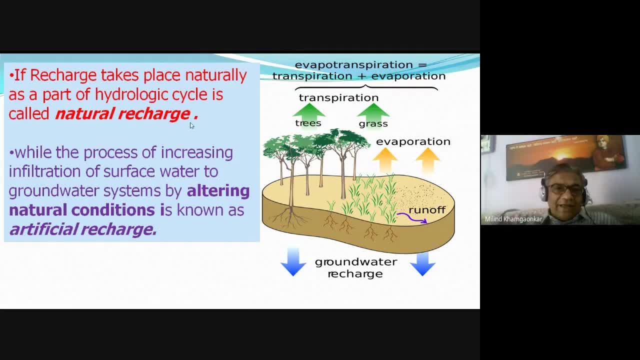 cycle way, then this type of the recharge is called as the natural recharge. okay, naturally, but sometimes we, this natural process, get disrupted due to the over use of the groundwater. then we need to recharge this groundwater. and then we need to recharge this groundwater, then we need to recharge this groundwater. 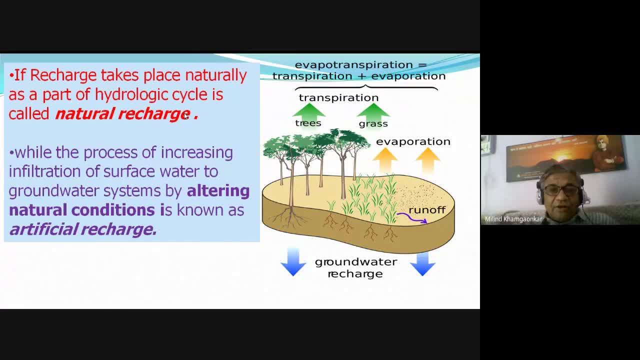 by additional human efforts, then the additional efforts, which are other than natural recharge methods, taken by the human beings, that is, the process of increasing this infiltration of the surface water to the groundwater system by altering or by changing certain natural conditions, is known as artificial recharge, and we are more interested in this artificial recharge. 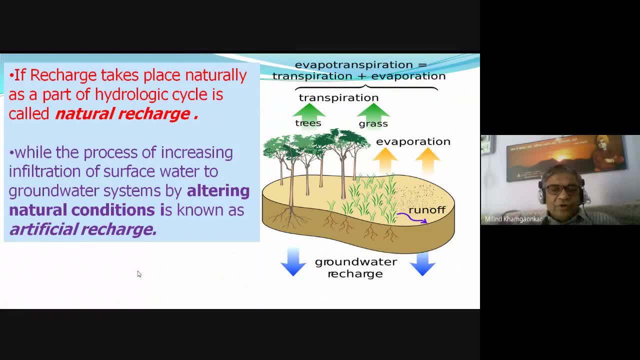 and a natural recharge locally at the grabsim. but when we are extracting more water than what is being naturally recharged- naturally recharged to check further- naturally the water contains more water and the system that is being produced leads the system to recover. then the system to recover, then the system to recover means everything. we are, he there, what we? We are basically exploited for this water, and now we're not speaking of- and roughly speaking about this to everything working on the land of which it is不要大家. 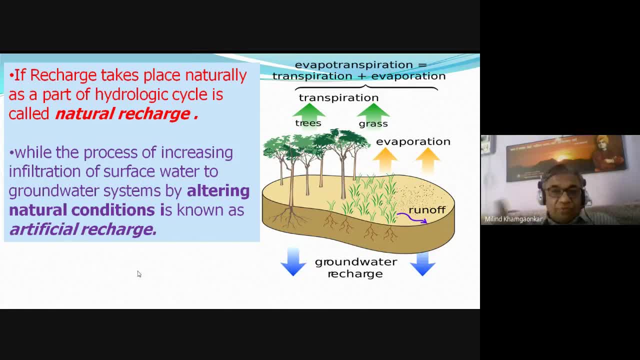 Then those aquifers needed to be artificially recharged Again. artificial recharge karne ke liye koi hum khud tori proper water produce karte hai, Again by altering certain natural conditions. Jo bhi rainfall aata hai, usko hi firse ham reutilize karke kaise aur use karenge Ya kahi paani bekar bahe jata hai, nadi me se Samandar me jata hai. Toh all that water is to be used for the recharging purposes by altering, as has been said here, certain natural conditions. 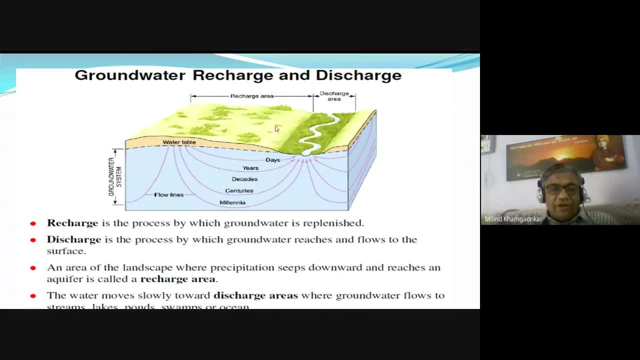 Through this photograph again, you will be very well understand How. what is the recharge and what is the discharge? Recharge is the process by which the groundwater is replenished and refilled or recharged. Replenished means refilled or the recharged. 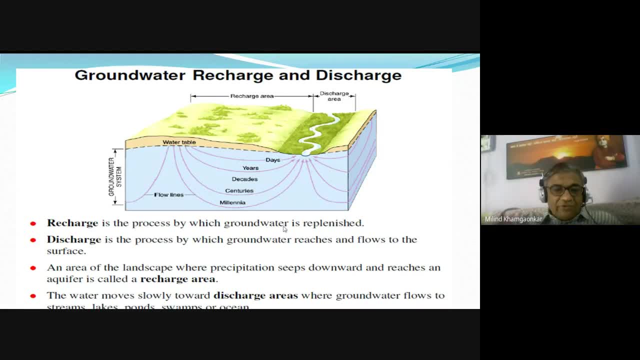 So it is called as a recharge, by which the groundwater is replenished or refilled, And discharge is the process by which groundwater reaches and flows to the surface Groundwater, when it is taken out either by the pumping to the surface of the soil or when it reaches to certain streams. when the groundwater table is above the river bed level or the stream bed level, then this groundwater is being supplied to these streams. 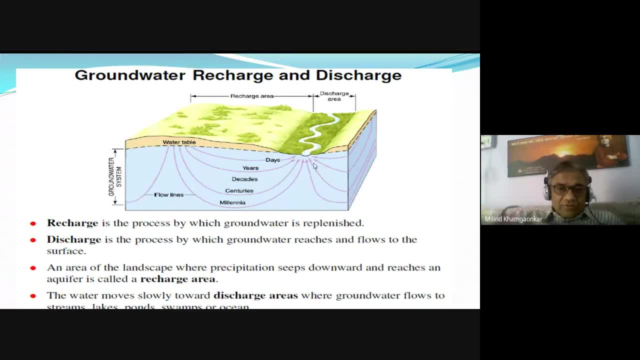 Then also this: we lose certain groundwater. That is called as the discharge, Then the recharge area, An area of the landscape or the soil or the topography, The area of the landscape where the precipitation seeps or percolates or infiltrates downwards and reaches an aquifer, is called 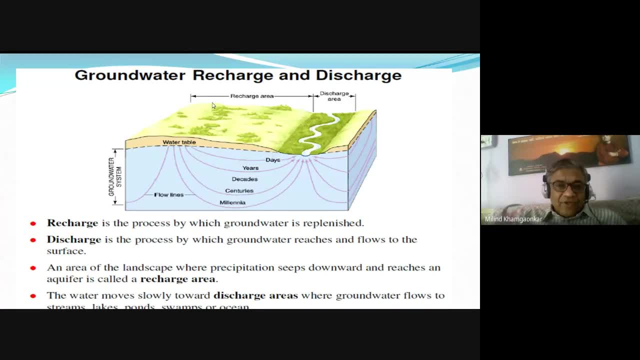 As the recharge area, as has been shown here, and the stream area or the river part is called as the discharge area. recharge area and the discharge area The water moves slowly toward. discharge area where groundwater flows to the streams, lakes, ponds, swamps or the ocean. 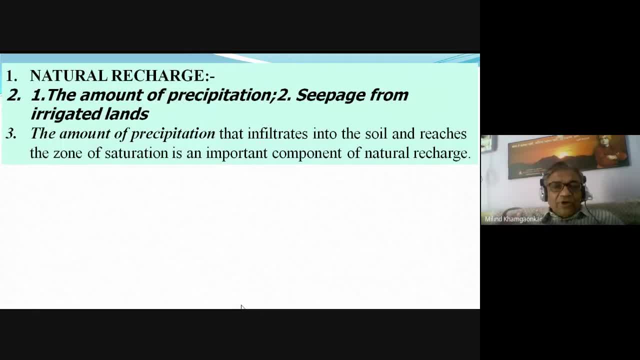 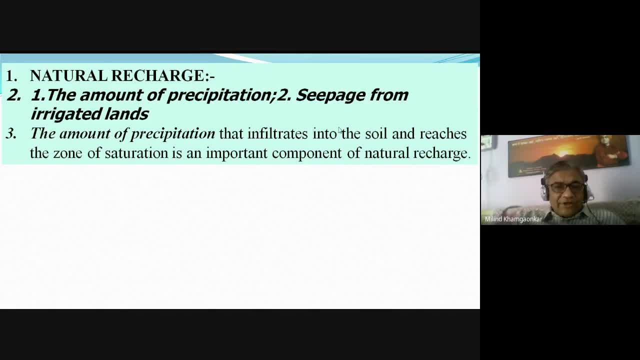 So whatever part or percentage of the precipitation, So whatever part of the precipitation, Rainfall, When it percolates into the soil and moves downwards towards the aquifer via infiltration, via percolation by the gravity pressure, gravitational force, 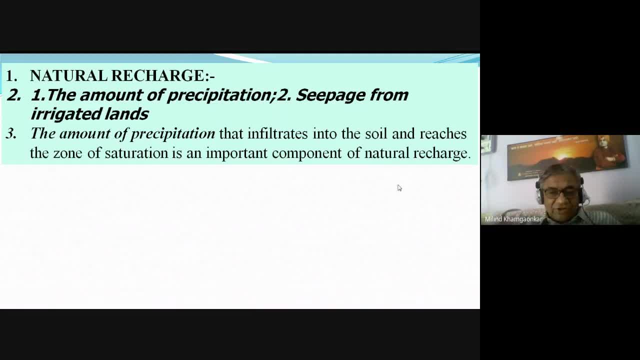 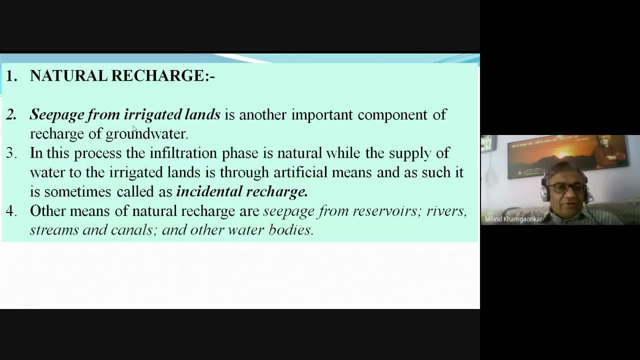 And reaches to zone of saturation is called as the natural recharge. in natural recharge there is another type of the recharge, that is recharge from the irrigated lands, sometimes through the dams or through the wells. we supply water for the agriculture purpose on the land, then this water hundred percent is not utilized by the plants nor. 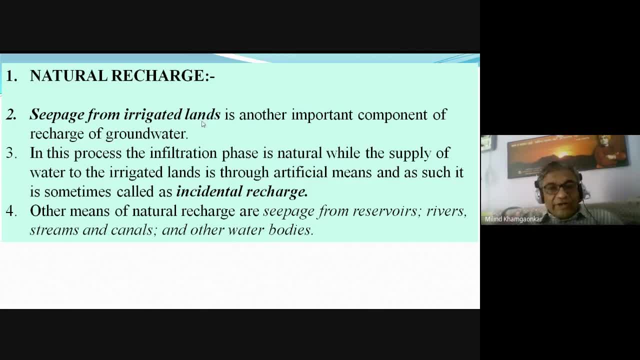 it gets evaporated, but some water percolates into the ground and again recharges the ground water flow or the aquifer. this type of the recharge is called as the incidental recharge, in which the infiltration process is a natural process, only the supply of water is not. 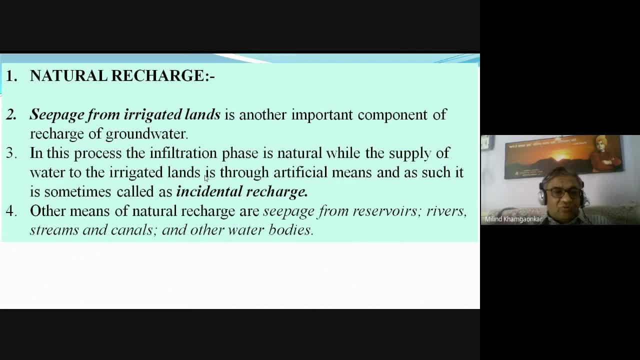 by the rainfall or precipitation, but it is the irrigation water through the soil. though we supply irrigation water by artificial means, that is, through canals or through pumps through the well, but such type of the recharging is called as the incidental recharge. you know one of the 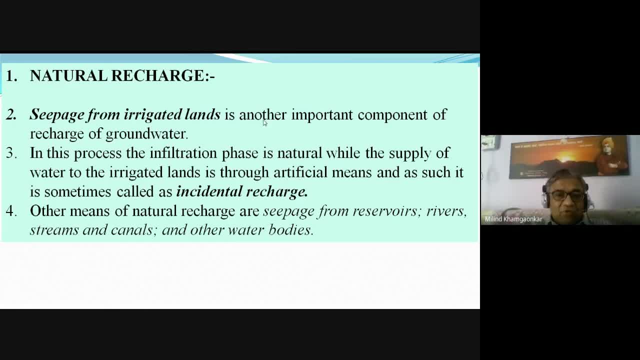 definition. sometimes they may ask into the exam what is incidental recharge? other types of the natural recharges are the seepage from the reservoir, that is, the dams or the tanks or the ponds, seepage through rivers. river is nothing but the flowing channel through. the streams are smaller than the rivers. 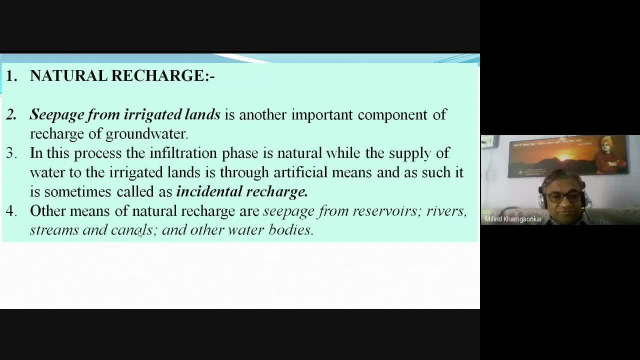 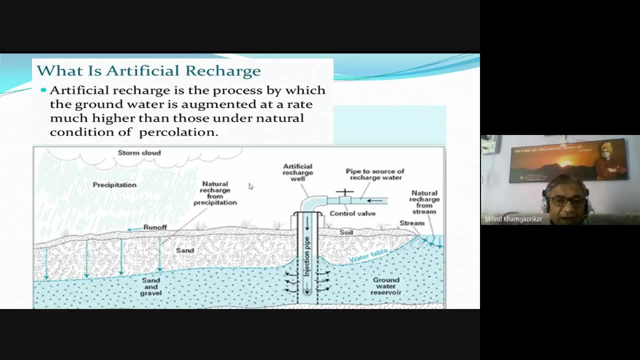 small Nala's canals, the irrigation canals and other water bodies like the ponds, etc. so these are all these. all comes under the natural recharge. now, what is artificial recharge is the process by which the groundwater is augmented, that is, supplied or refilled at a rate much higher than those under. 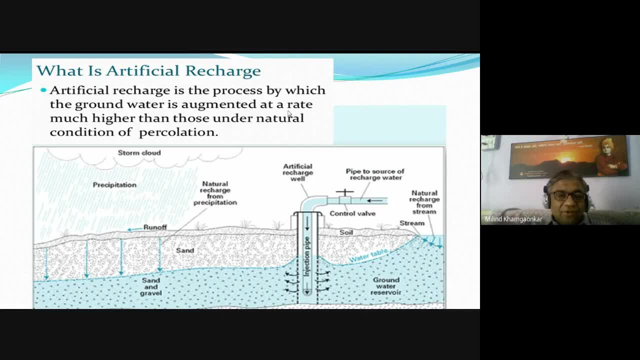 natural condition of percolation. so when we recharge artificially, then that recharging is much faster than the natural recharging wherein the groundwater, which may be in the aquifer of confined or unconfined type, is directly supplied with the water and these both these aquifers are refilled with the water or recharged. but this all 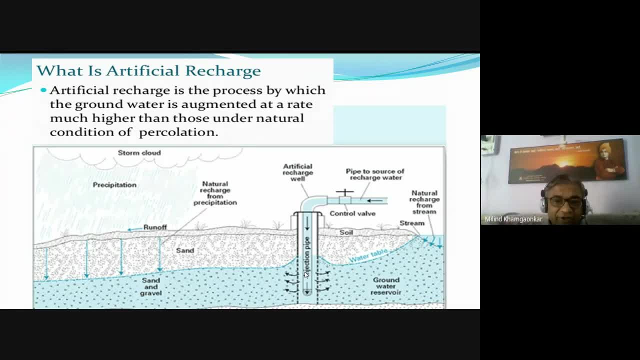 process occurs not naturally, not through the natural precipitation or rainfall and the percolation of the water. so this is the natural recharging process and the percolation or the infiltration, subsurface, sub groundwater flow or the base flow, not through that hydrological cycle process but other than. 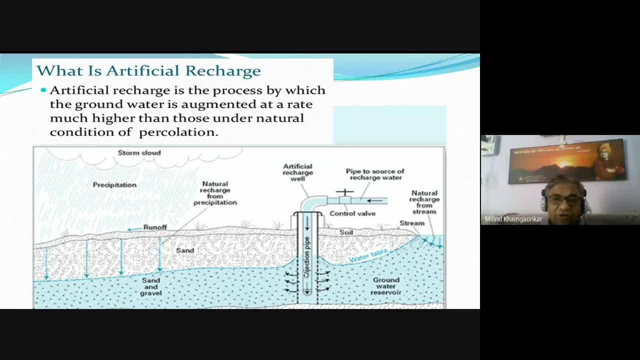 hydrological cycle and other than the irrigation or the incidental recharge, by supplying the water through the wells, by supplying the water through the pipeline, etc. then such type of the recharging is called as the artificial recharge, and here you can see in this sketch wherein the natural recharge from precipitation is also shown. 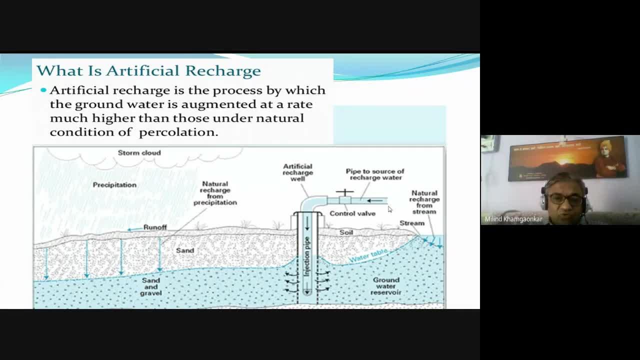 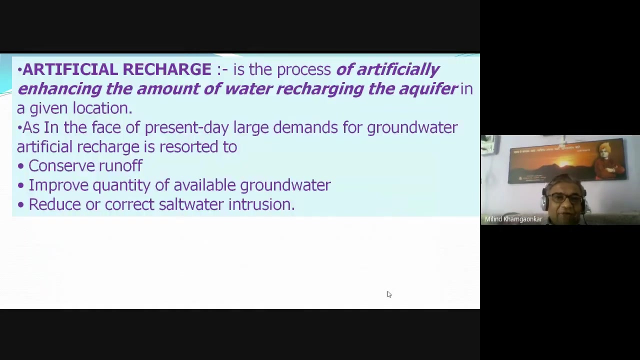 on the left side and the artificial recharge to the pipeline. the water is being for dw, site out, percolate through a recharge. well is being shown and this water is being percolated. things are irreversibly variable and the transferred through this aquifers. so artificial recharge is the process of artificial enhancing. 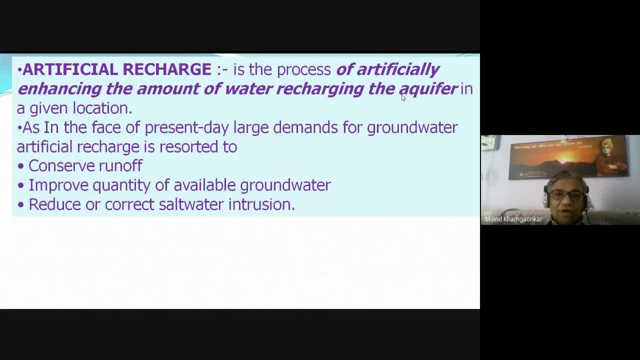 or increasing the amount of the water, recharging the aquifer in the given location, where we artificially, with the help of certain means, with the help of the pipes, pumps, etc. to the aquifer to enhance or to increase the aquifer water is called as the artificial recharge. 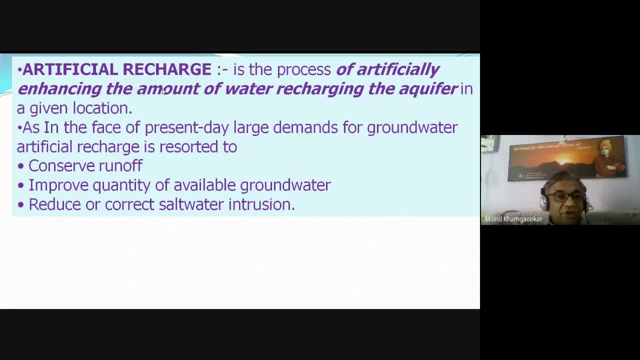 why artificial recharge is so important, why it has got so important- though it is a controversial subject or controversial issue- that our population is increasing in geometric proportion. our population is still at number 2 in the world, and by 2050 we will be at number 1. 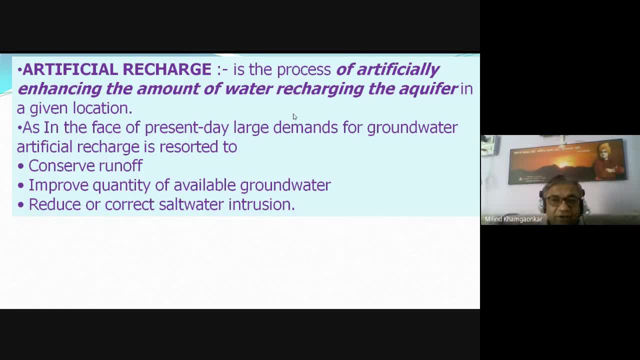 China is at number 1 and we will go further than that. so the population is increasing. the population is increasing, so people need water for drinking and for their regular use. you know, 150 to 200 liters per day is the WHO limits of the water requirement. 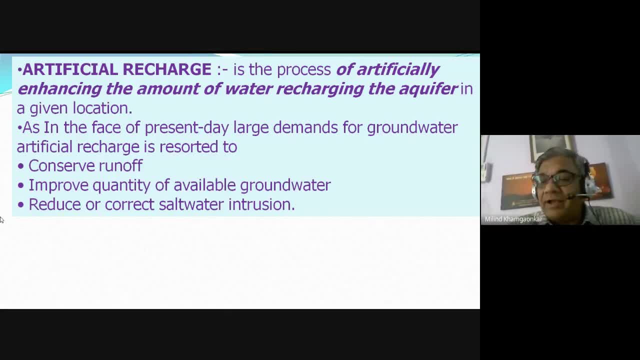 and the water is not only required for drinking and for the day-to-day consumption, but also what they need: certain food, they need the anage, and then for growing and for harvesting those crops also water is needed. so therefore, in present day situation, large demand for ground water is there. 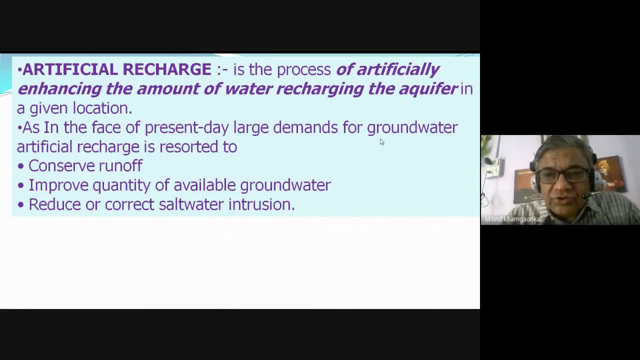 and as the source and the water availability is limited, there is very little water under the ground. if we take out as much as there is, then that water will be finished. so that's why artificial recharge is very important: to conserve the runoff- the runoff, surface runoff or sub-surface runoff. 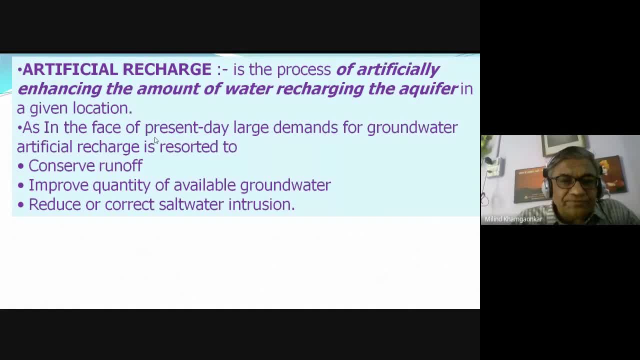 which flows to the river and then, through river, it goes to the ocean or to the sea and it is wasted. so that water needs that runoff, needs water, that that runoff needs to be conserved or saved somewhere. we do this and why we do it. we construct the dams. 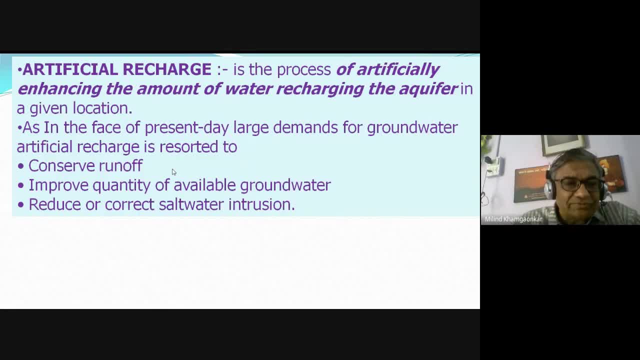 that water should be stored. or consider also by recharging the ground water also, we can conserve the runoff again. this ground water recharging is useful to improve the quantity of the runoff, the available ground water, as well as quality quantity we can achieve, as well as to improve. 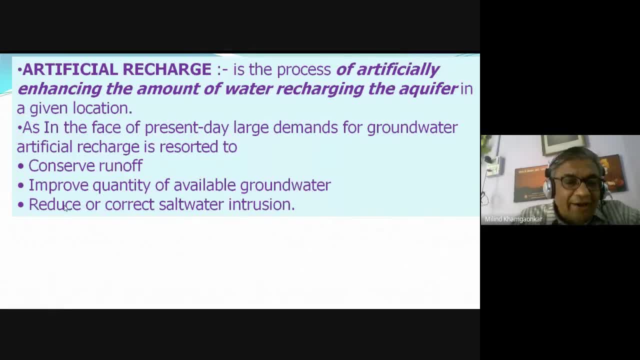 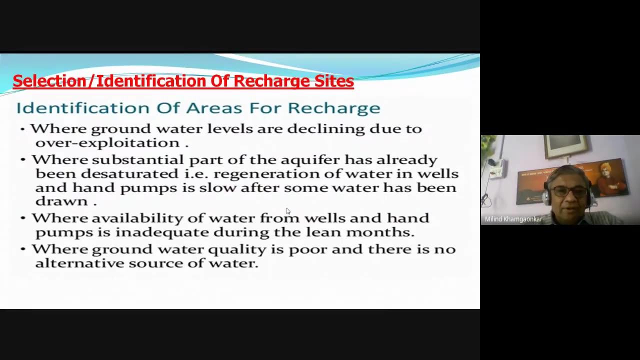 the quantity of the ground water and to reduce or correct the salt water intrusion, and the ground water will slowly reduce and the salty or saline water will increase. now, selection and identification of the recharge sites. sometimes it is asked in exam: how will we identify where to recharge? where to recharge? 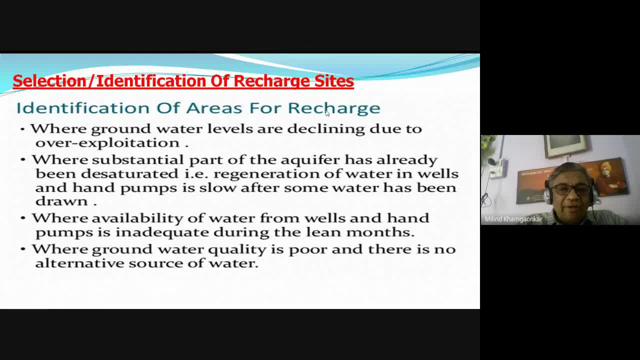 in which area to recharge, where the ground water should be, where the ground water levels are declining due to over exploitation, where the ground water table or piezometric surface- both are going very low. they don't go down on their own. nature never imbalances itself. 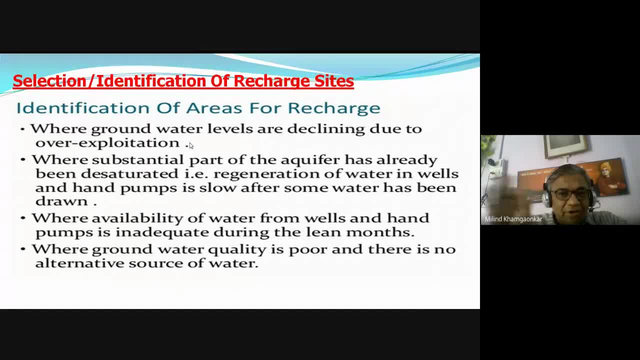 nature does not reduce the water table on its own, it does the reverse: recharging every year, naturally, maybe unconfined, maybe confined aquifer. we humans do that. we humans are playing with the nature. therefore, we are facing all these problems. one of the problem is corona. 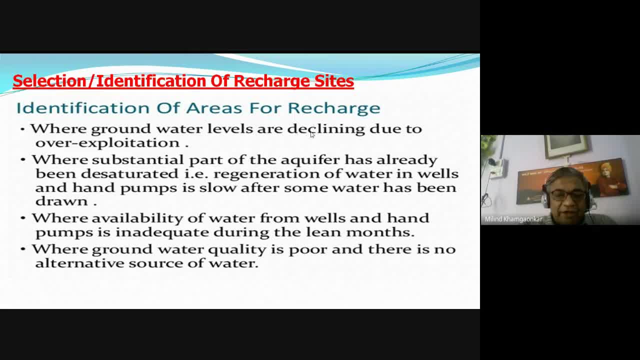 so we are exploiting the groundwater. i give you all example: There are a lot of orange gardens in Katol, Narkhed and Sauner and there is a cash crop of orange, so it also needs water. but the ground water is pumped from it and that is why the ground water table has gone down, so the piezometric head is also going down. 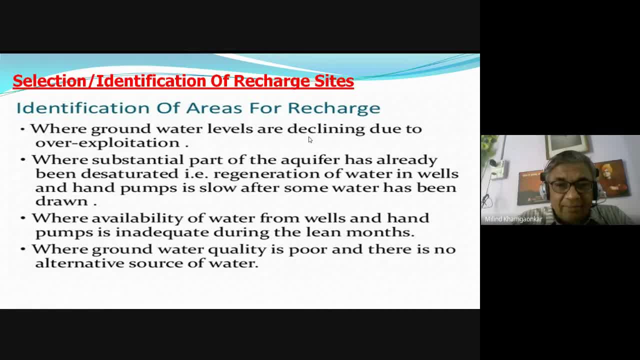 Now, if we have to bring it up again, what will we have to do? We will have to recharge it. So where do we have to recharge it? Where the ground water level or piezometric surface are declining due to the over-exploitation. exploitation means overuse, over-pumping out where substantial part of the aquifer has already been desaturated. 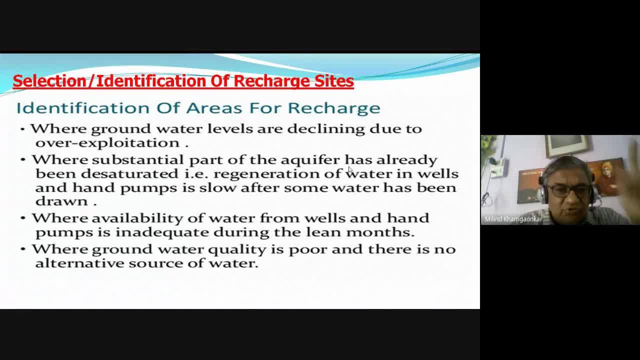 That is, the regeneration of water in wells and hand pumps is slow after some water has been drawn. When the water from the aquifer is depleted, then the well- maybe an open well, or maybe a bore well, or what is called a hand pump. 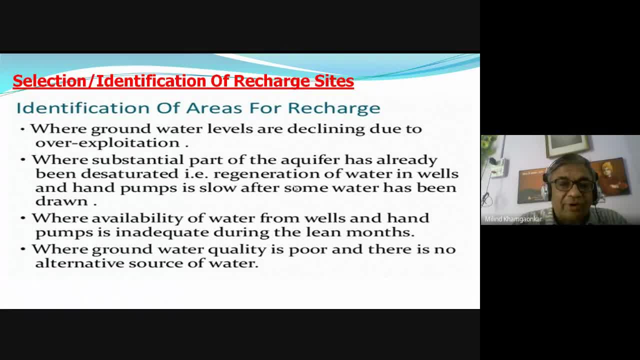 it takes a lot of time for it to recharge naturally. It may take years together to naturally recharge and to bring it to its original groundwater availability. So therefore, here, at such locations where the aquifers have dried, there this recharging is necessary. 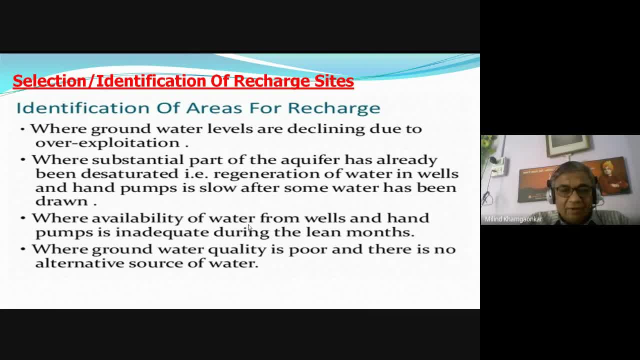 Thank you. And where the water? in the extension of this again, where the water availability from the open wells as well as hand pumps is inadequate during the lean months. Lean month means the monsoon season, Or lean means in which there is less amount of water, in which lower quantity of the water is available. 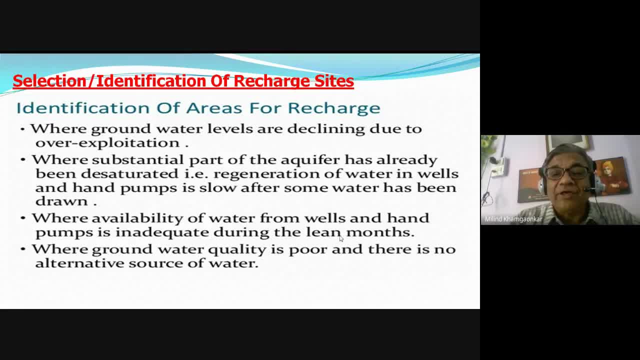 Lower quantity. Lean means lower quantity. you can say Lean month means where the quantity of water is available in lesser units. And when this happens, This happens in the summer. In the monsoon season there is no water in the wells and hand pumps. 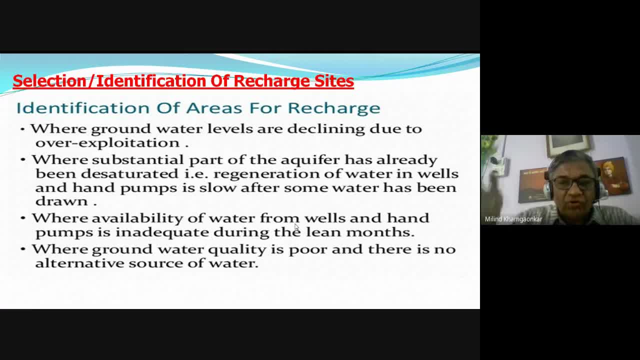 You see on TV that people are getting down from the well, taking out water from the well, filling buckets of water and using that water. We brought this situation. Nature has not brought this condition. We have over-exploited the groundwater. Therefore, in summer we have to run, helter and shelter for the drop of water. 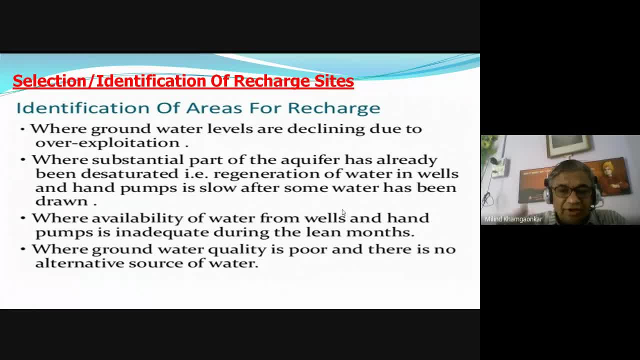 Right. Some of you who have less rain in the area must have this problem In the monsoon season. to bring water, we have to roam around here and there, So we will recharge in this area And where groundwater quality is poor and there is no alternative source of water. 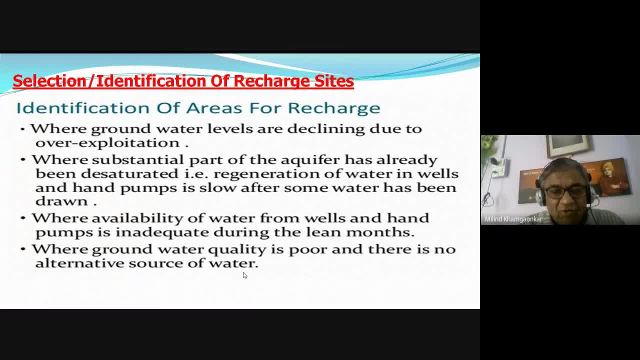 We have a lot of areas here In Akola district or somewhere in Malkapur or in Buldana district All along that Purna river, some part of that Purna river, the saline belt is there- Or some other areas in our district of Gadcharuli. 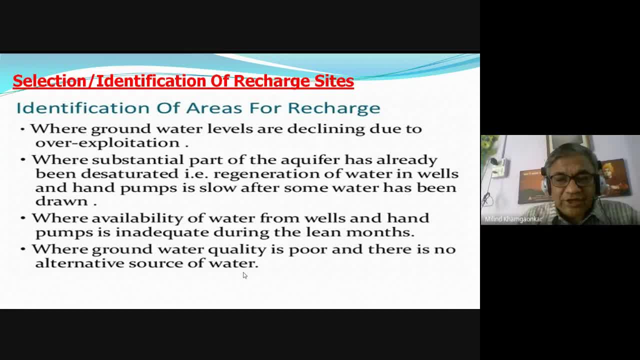 There is saline and there is a lot of fluoride. So if we have to reduce their intensity and quantity, we have to recharge the groundwater there, So it will improve the groundwater quality. So at all such locations, at all such areas, 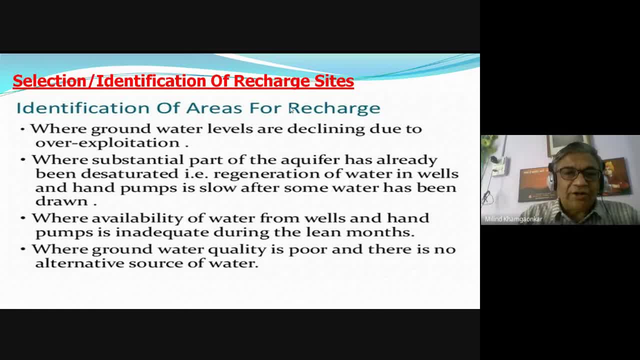 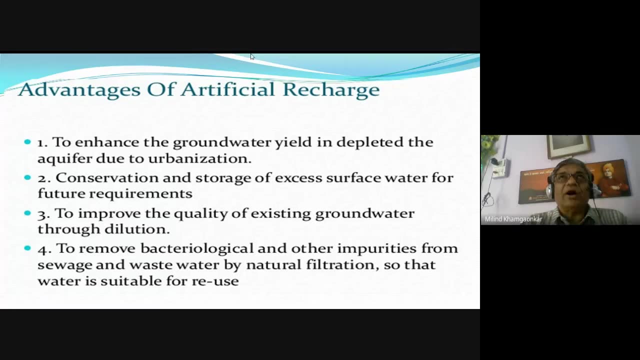 we needed, on priority, the groundwater recharge, So such sites to be located and then identified And then the recharging of the groundwater is to be planned there. What are the advantages of the artificial recharge? To enhance the groundwater yield in depleted aquifer due to urbanization. 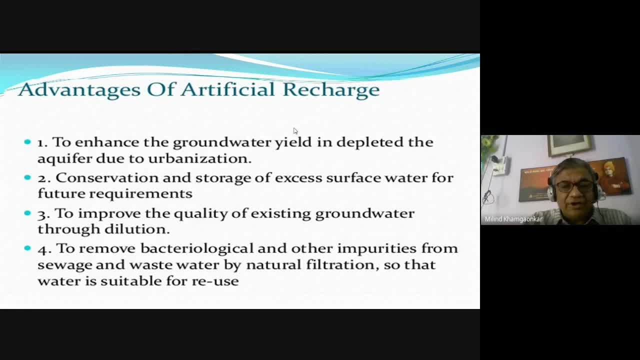 Enhance and increase the groundwater yield Yield in a water that can be taken out. So to enhance or to increase the groundwater yield which is already depleted, which has already decreased into the aquifer due to urbanization. That is urbanization. 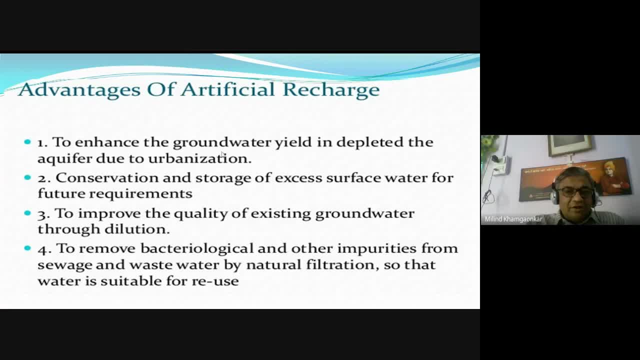 By urbanization the groundwater in the ground has been removed a lot. Conservation and storage of the excess surface water for future requirement. Surface water, the surface runoff. it flows into the river, goes into the sea from the river and becomes waste. 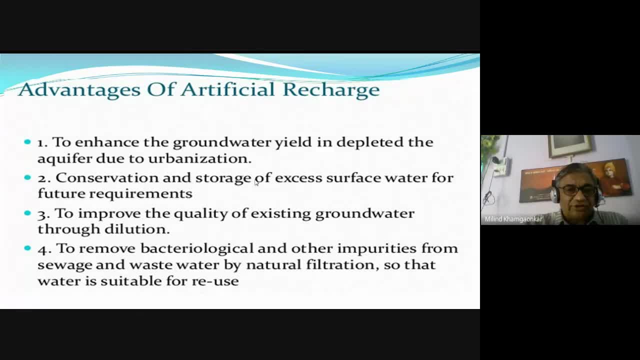 So to preserve and store it. we have to conserve and store it For this. these are the advantages of artificial recharge: To improve the quality of existing groundwater through dilution. Existing groundwater, suppose there is some salt in it, there are some fluorides in it, there are some chlorides in it. 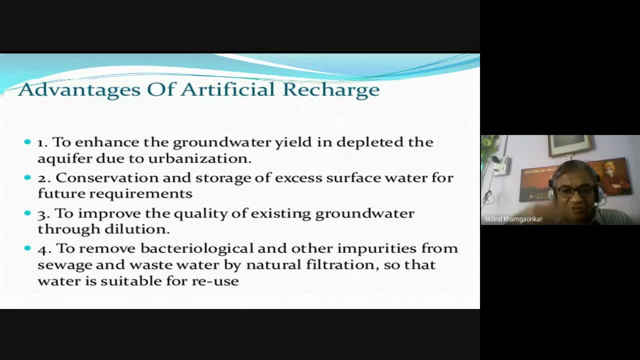 or some other material which is dangerous for the human health. that can be improved by percolating the fresh rainwater To remove the bacteria, logical and other impurities from the sewage and waste water by natural filtration so that water is suitable for reuse. 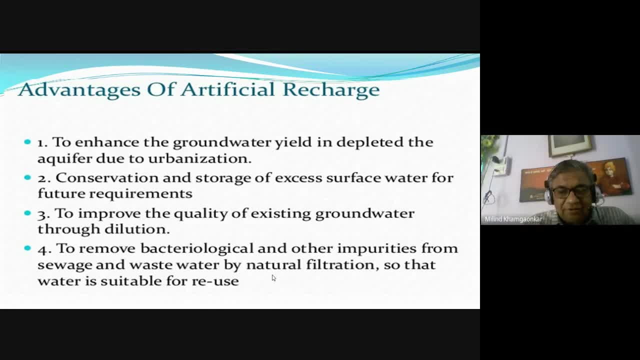 The wastewater, like the lakhs of liters of water in Nagpur, is prepared every day. What do you count? There are 10-15 lakhs of the population of Nagpur. Every person uses at least 100 liters of water daily. 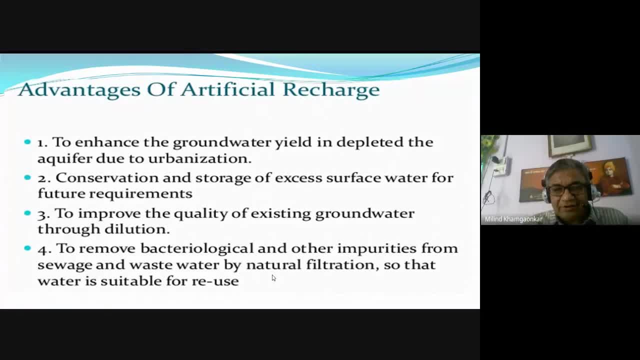 Take 50% of that wastage- 50 liters, So 15 lakhs. multiplied by 50 liters Approximately it comes to 7-75 lakhs. So this much water is wasted from the Nag river. It is called Nag Nala. 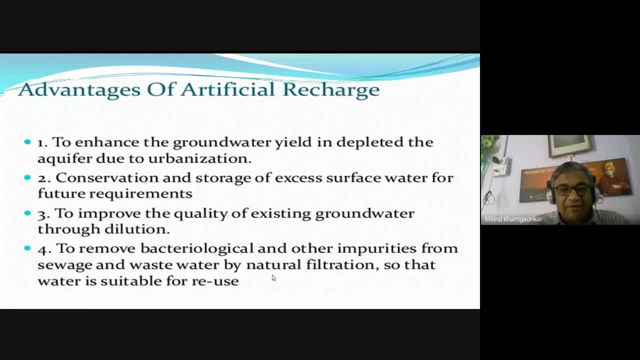 So what is the reason? In Bhandewadi there is a wastewater treatment plant And from this wastewater good water is separated out And it is used in the Koradi thermal power plant. You know, or I don't know. 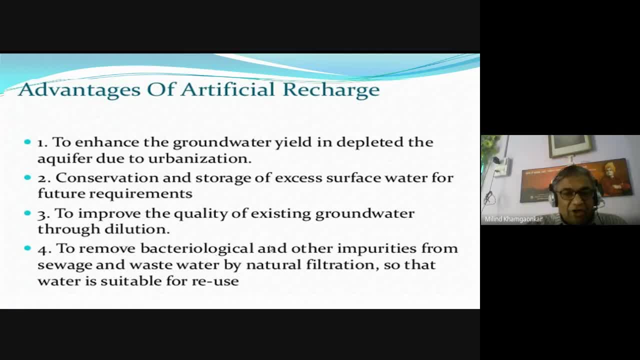 So again, by removing the bacteria, the bacteriological and other impurities from that sewage, that is the wastewater, by the various treatment methods, and that water can be reused for the recharging, also artificial recharge- purpose. So these are the advantages of the artificial recharge. 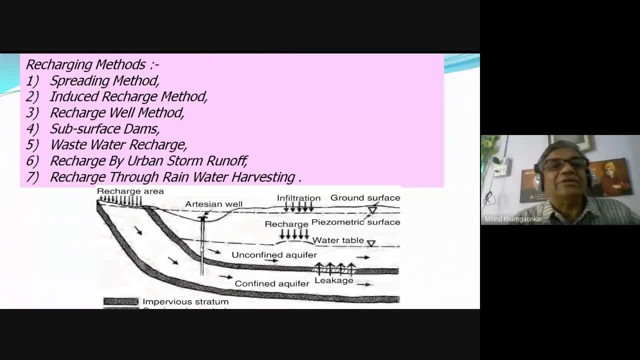 Now we will move on to the various recharging methods, Isn't it So? recharging is a very important method which is also in our syllabus And on it once or twice or regularly every year on some or the other method. 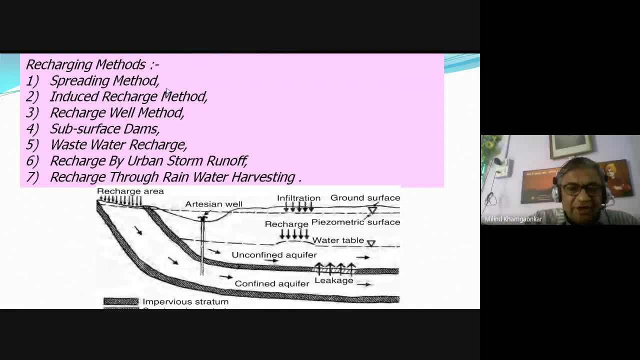 there are notes, short notes. We are reading it very well, in detail. We are understanding one thing, But according to the exam, according to the marks allotted to that question, you have to write down your answers. So recharging methods. 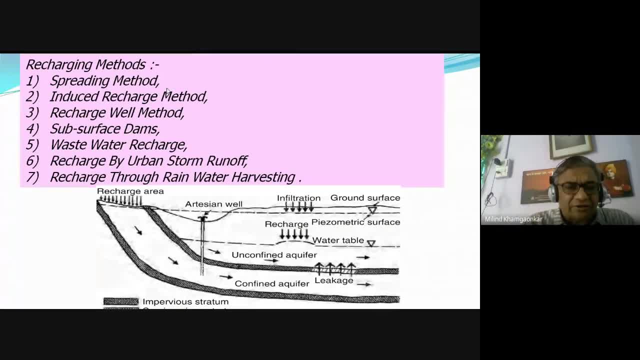 Seven main methods. There are numerous methods, But seven out of that methods are being taken for our study. The first is the spreading method. The second is the induced or indirect recharge method. Third is the recharge well method. Fourth is the sub-surface dams. 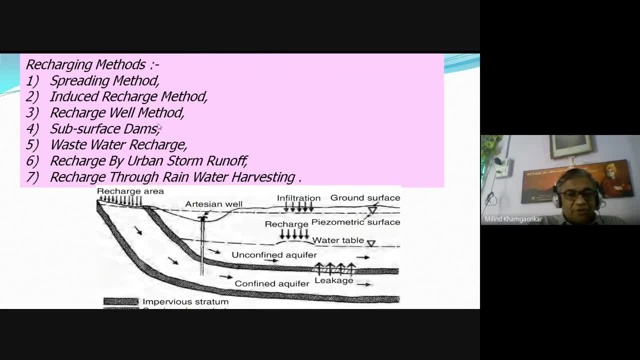 We have seen the dams above the surface, But we can also do something under the surface of the ground, like a dam, which will be helpful for increasing the groundwater flow or the groundwater recharge. So sub-surface dams, Wastewater recharge. 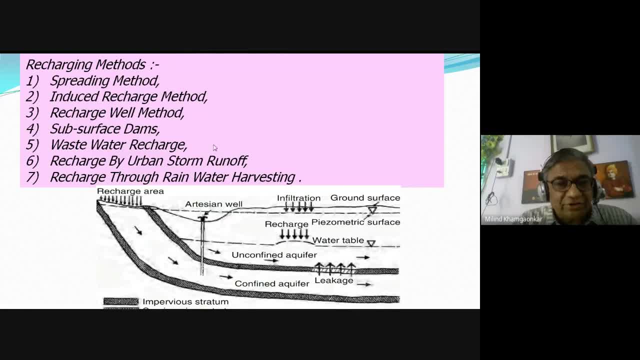 As I have just told you, Nagpur produces more than 75 lakhs of the wastewater daily And that water is being wasted through the Nag Nala, etc. Some part is being reused for the Koradi thermal power plant, So that wastewater recharge is very important. One of the methods of the recharging of the groundwater: Recharge by urban storm runoff. The type of rainwater in the city or in the city, The type of rainwater is recharged by the urban storm runoff, And recharge through rainwater harvesting. 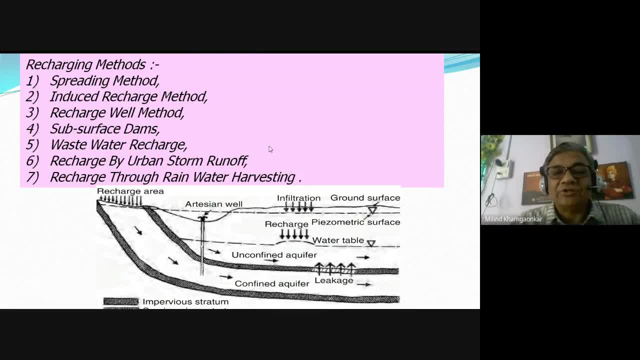 Which is an independent point to be discussed Again. with the help of certain sketches I tried to understand you. That again, this is the ground surface. at the top, Precipitation occurs, Some water infiltrates To the unconfined aquifer. 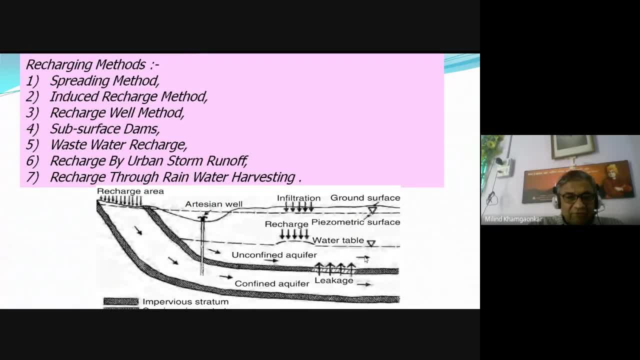 And the water into the unconfined aquifer increases In the form of the increase in the water table, groundwater table. Also, through certain recharge areas Where this confined aquifer meets to the ground, Cross section that area, Which is a percolated area. 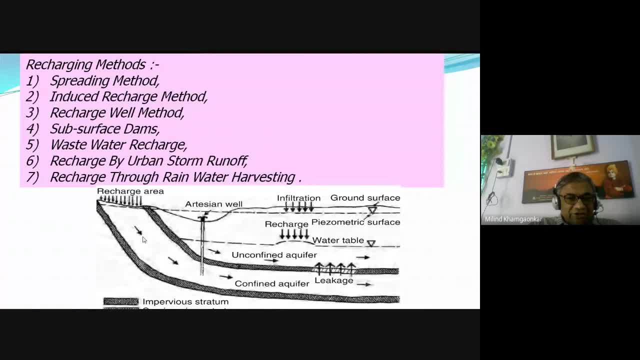 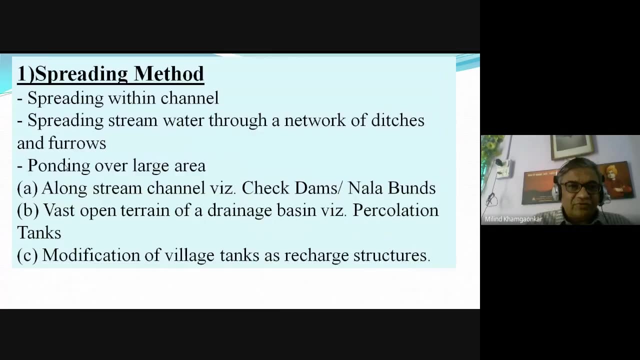 Which is a permeable strata Which recharges, or the water through it is reached to the confined aquifer. So all this is being recharged, So all this is being taken out through all these seven methods We will discuss one by one. 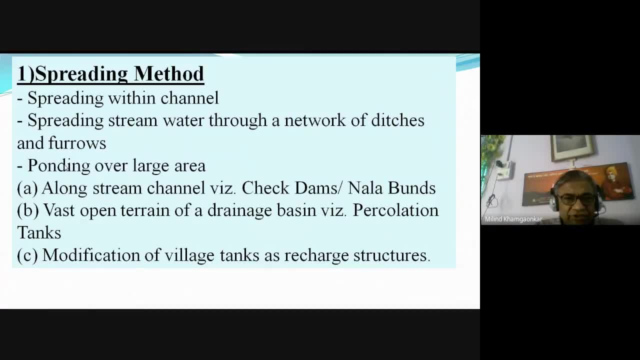 The first is the spreading method. As the name suggests, The water which is available May be a Rainfall water, Or may be a water into the channel, Or may be a water into the stream, Or may be a water into the river. 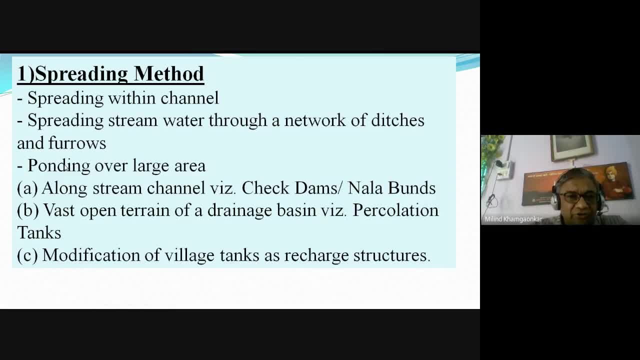 Which, if not conserved Or preserved Into the groundwater, Then it will be wasted into the sea. Ultimately, all the rivers Meet to the sea, All the rivers meet the sea And after going into the sea, Then it is not reusable. 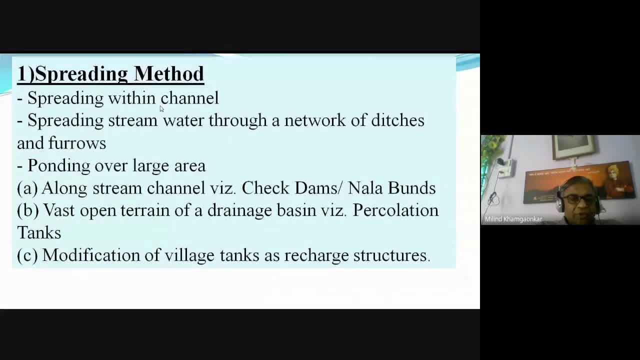 So what is done in the spreading method? That the channel or the river May be changed in some way or the other in the river So that the entire water does not flow into the sea. So spreading within the channel, Spreading stream water. 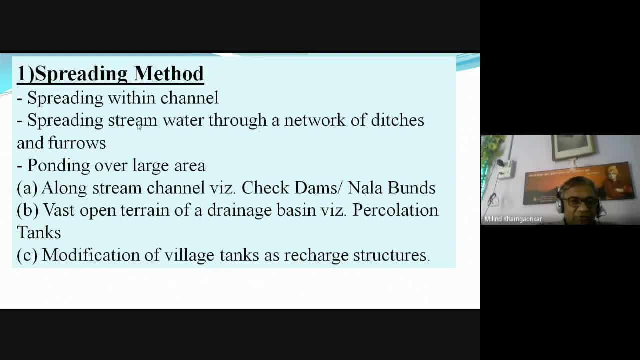 Through the network of ditches and furrows, The water of the river. This is the water of the river Next to the river. By making some drains, Which we will call ditches and furrows, By excavating certain Ditches or the furrows, 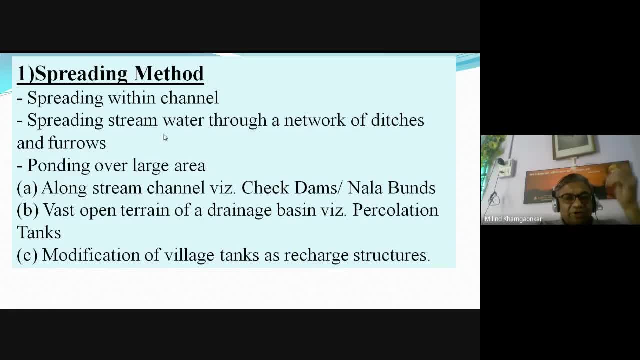 Or by excavating certain pits, Pits. Pits can also be dug And this water of the river We will bring and leave in it By gravity, Not by pump. Then it will not come full To take it from the pump. 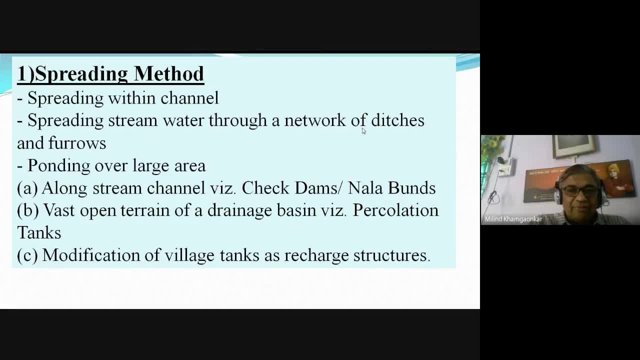 So we will take it from the gravity And the pits which we have made, The drains which we have made. We will leave this water in it So that it will percolate in the ground And increase the ground water table. 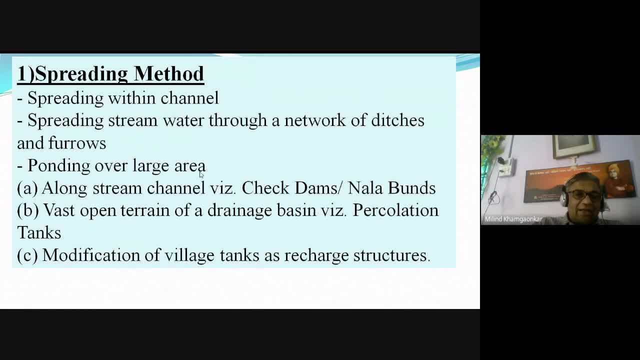 So that is the second method. Third is the ponding over the large area. If we have a lot of land available, Then above it This rainwater, We will stop it in it And then we will let it percolate in the ground. 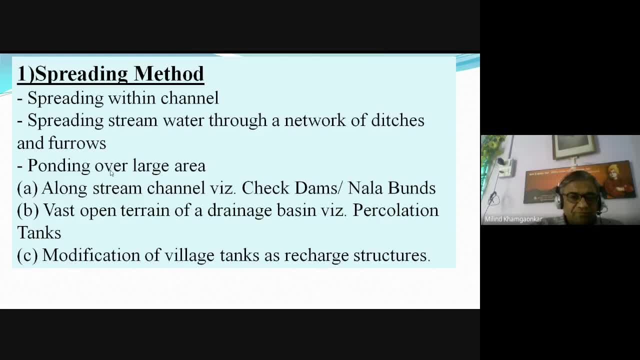 And then we will let it percolate in the ground. This is being achieved Through, again Through sub methods, That is, the along the stream channel And a river Which flows By constructing some obstructions in it, Like the Cheikh Dams. 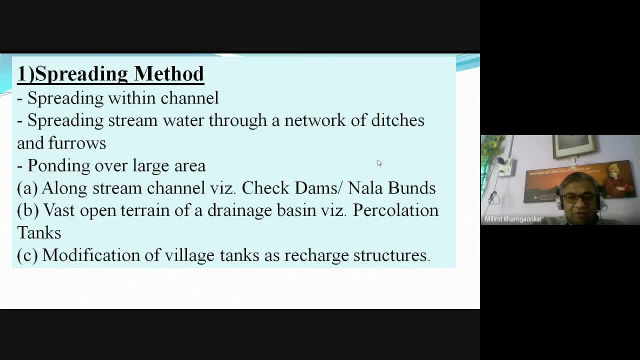 The Nala Burns. The water is being obstructed To flow To the sea or the ocean And that obstructed water is being percolated or infiltrated into the ground Again. one of the spreading method. Another is vast open land or terrain of the drainage basin. 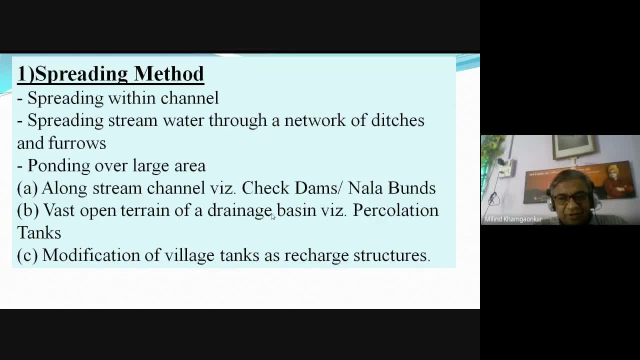 Via percolation tanks. If the catchment area is very large, Then a pond is constructed above the river or the drain, Which is called percolation tank, And if the water is stopped in that pond Then that water will be percolated. 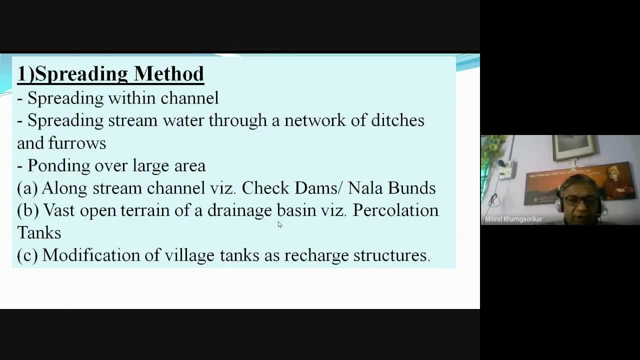 And ultimately That ground water table Or through the piezometric surface Will increase the piezometric head Through the percolation surface. And another third method of the spreading type is Modification of the village tanks, As rich as structures. 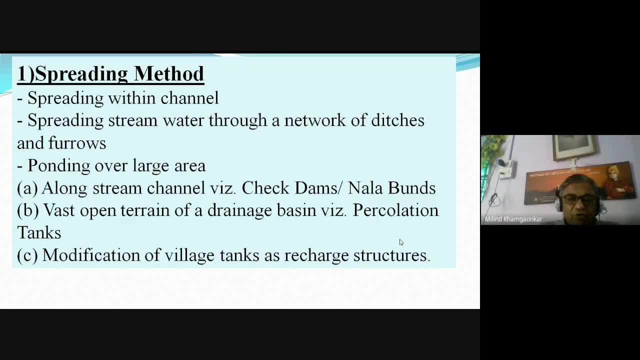 In your area, In the area of people, Your area, Bandara Chandrapur, Gadchiroli, There is a pond. in every small village It is called Bodhi. in your area, Bodhi Bodhi, Or in English it is called Maji maal guzari tank. 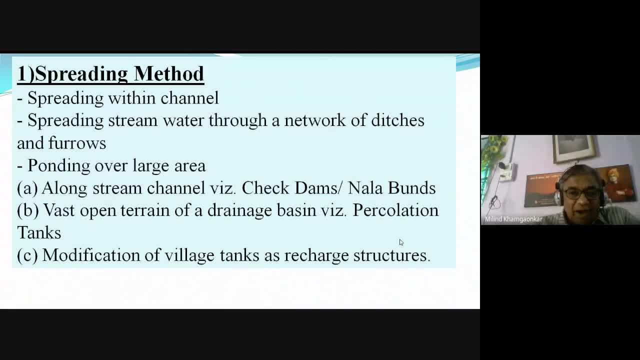 Maji maal guzari talao. It is also called Maji maal guzari tank. It is in your area, You know. Or in your local language, It is called Bodhi Bodhi, Or in our technical language: 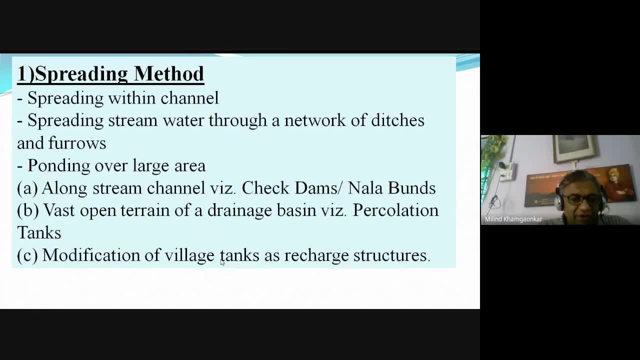 We call it village tank Khede ke talao, Small ponds in small villages, Constructed by our government Again To make available the Water resources. So this pond, This pond, In it The silt, That is called ghadu. 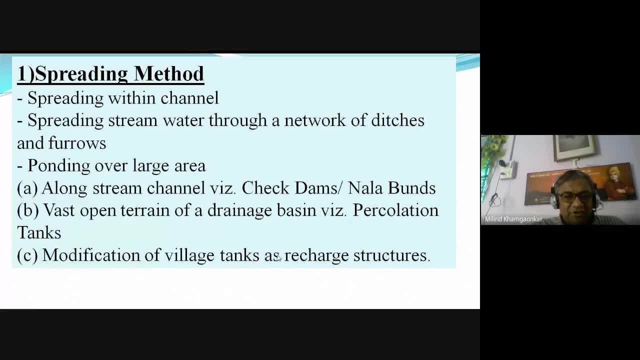 In it There are big pits Made of wells. The wells Are the ways, If we create, Which will Allow To percolate the water Into the ground And again Reach to the Reservoirs Or the aquifers. 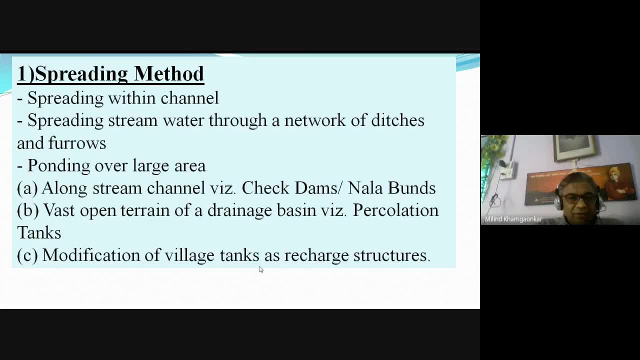 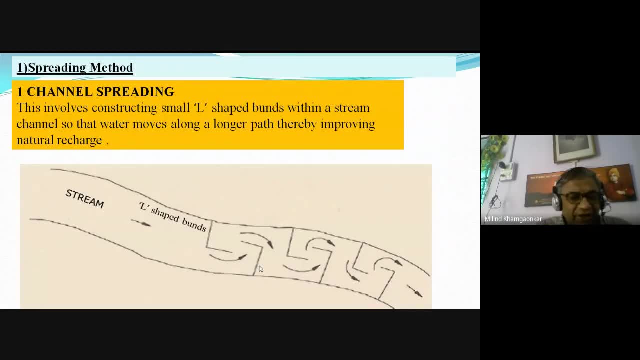 And will recharge. These are the Some methods of the Covered under Spreading method. There are two or three methods we can understand from this. The first method is channel spreading. Channel means stream, river or a well: How to stop the water in the channel, how to spread it so that the frozen water percolates in the soil. 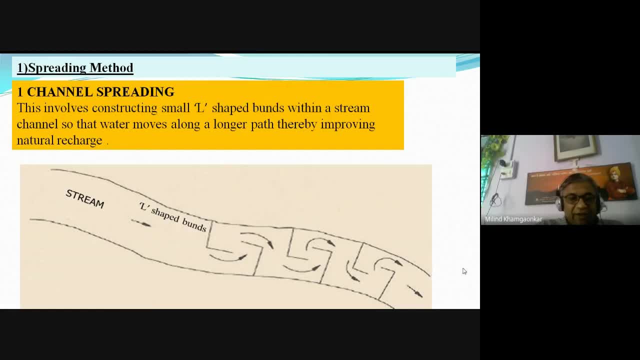 If it is not stopped, then it will flow from the stream, It will go from the stream to the big stream, from the big stream to the big stream and in the end it will go to the sea. So what do we do for that? 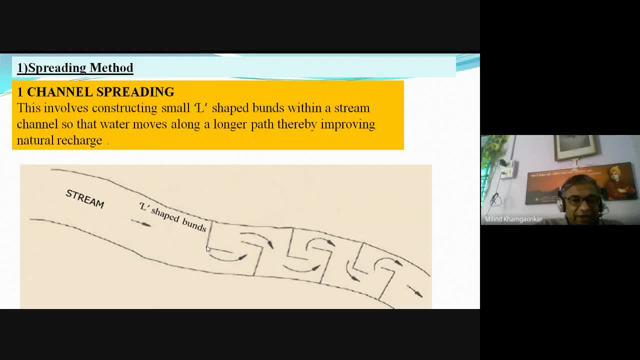 These rivers are made in the length of the river. Along the length of the river or the stream, The L-shaped bundles are constructed As shown here into the sketch. Bundles are nothing but the obstructions or the walls. Maybe these obstructions may be of the concrete or the masonry, or maybe soil made up of the soil. 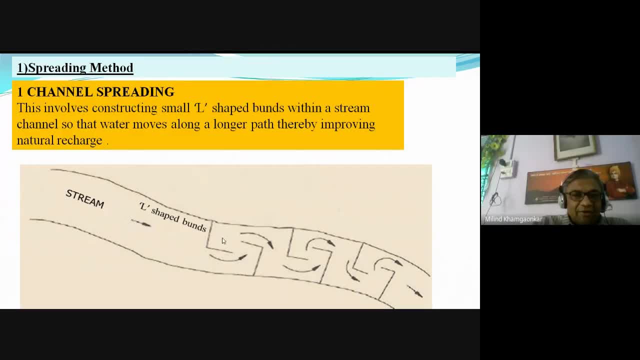 So they will be constructed so that, while the water is flowing, the water that is flowing from the stream. it will require more path, It will require more length to move from one place to another, And it will take more time into the stream. 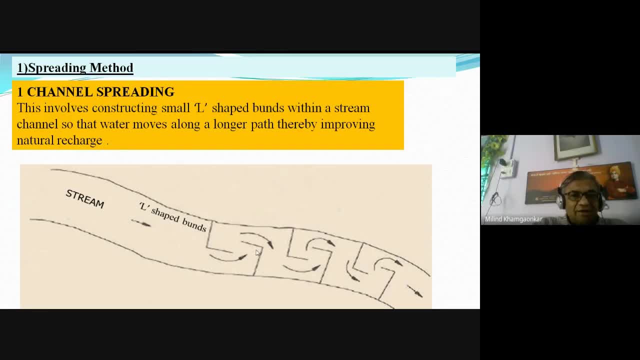 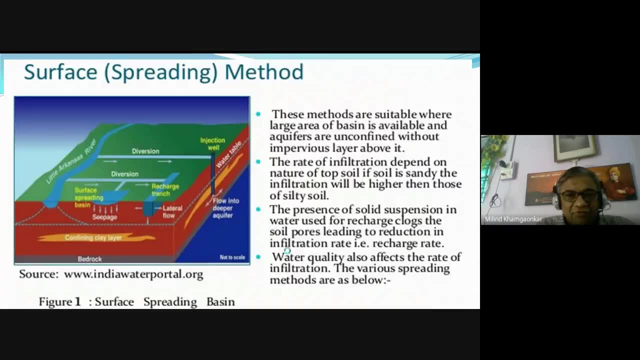 It will take more time to stay in the river And because of that the percolation will increase and natural recharge will be achieved. Then again, another method. The first is the channel spreading we have discussed. Another method is surface spreading. What is done in this? 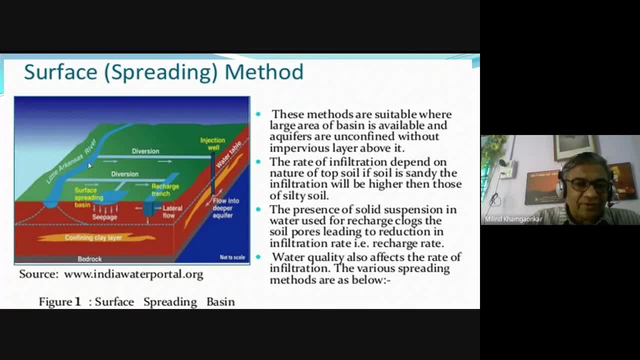 Like this is a stream, a river. From this flowing river, either perpendicular to the stream, some ditches or some furrows. These are excavated from the river, From the river, Through these ditches, through these furrows or peats. 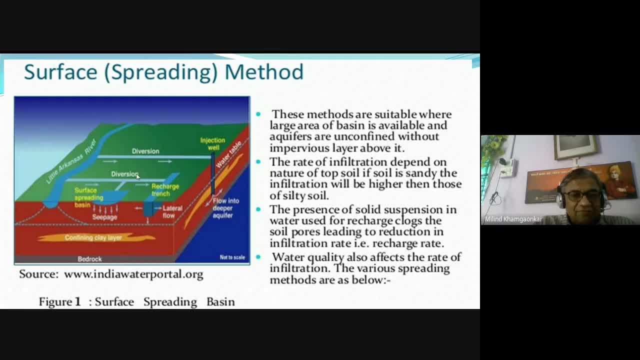 the water from the river is taken out And then it is brought over the land, over the surface other than the channel or the river surface. Either it is stored into the small ponds or small reservoirs, And it is also injected into the wells. 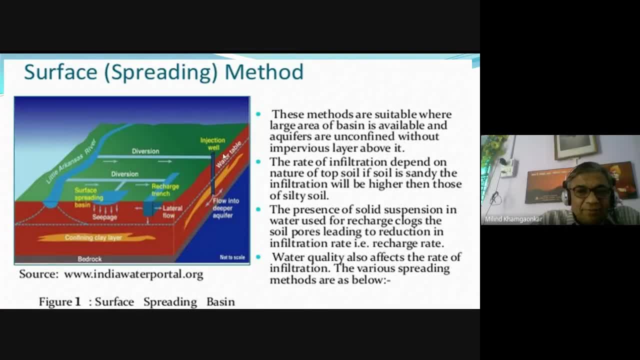 Whatever these diversion trenches are: Diversion trenches, diversion peats, diversion furrows- These are two or three words For the drains. They are called pits But furrows, diversion streams etc. Which are constructed or which are excavated perpendicular to the regular flowing river. 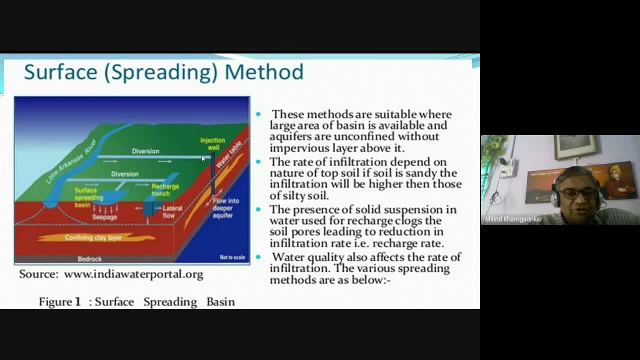 Water is being taken out through these furrows And is being allowed either to be accumulated in certain small ponds Or certain recharge trenches are again excavated perpendicular to this main trench or main furrow, Or this water through these trenches or these furrows. 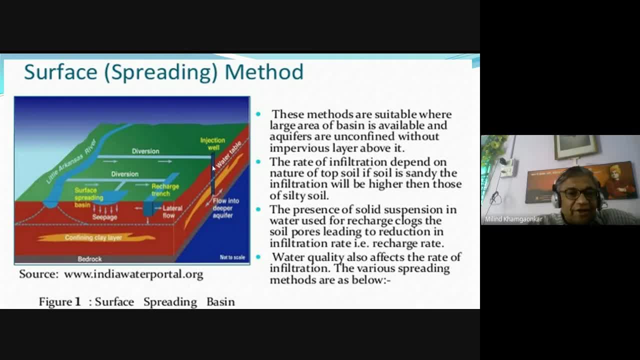 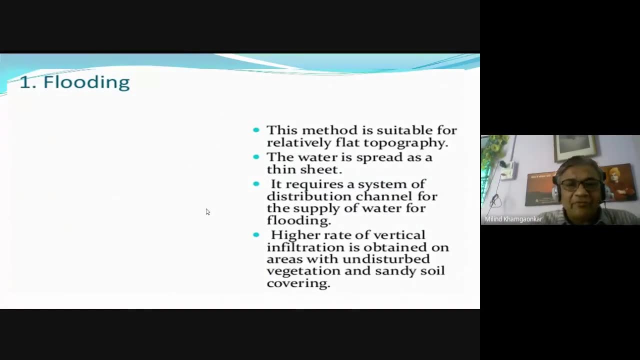 which is taken out from the river is injected into the well. It is left in the well, Which will reach to the ground water and recharge to the ground water table. There is another method wherein this water is being flooded Over the land.